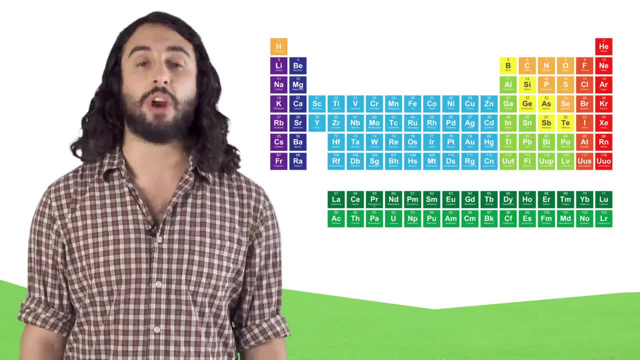 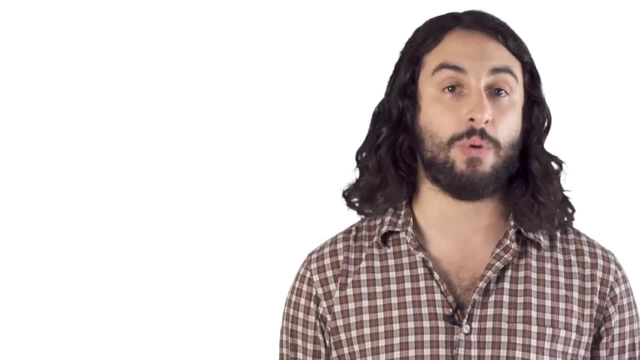 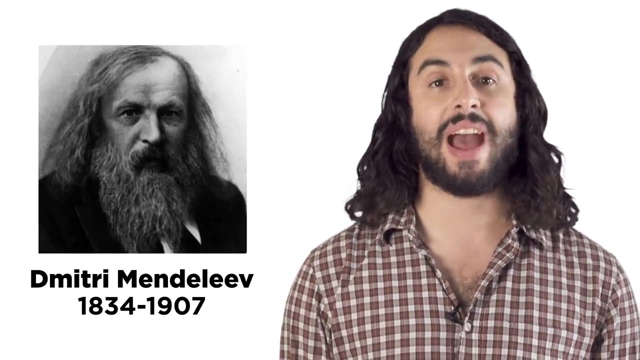 arranged, reveals many beautiful patterns that tell us about how nature operates. in the mid-1800s, lots of chemists were trying to come up with a way to depict all the elements in table form, and many different formats were proposed, but it was the one by Dmitri Mendeleev that stuck because of how well it correlates. 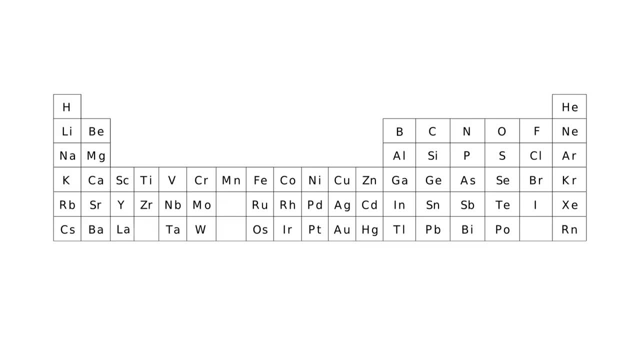 data as well as its predictive powers. he arranged the elements into rows called periods, and columns called groups. elements that had similar behavior were put in groups together, which helped to correlate existing data, and it also predicted the existence of elements that had never been seen before. with the 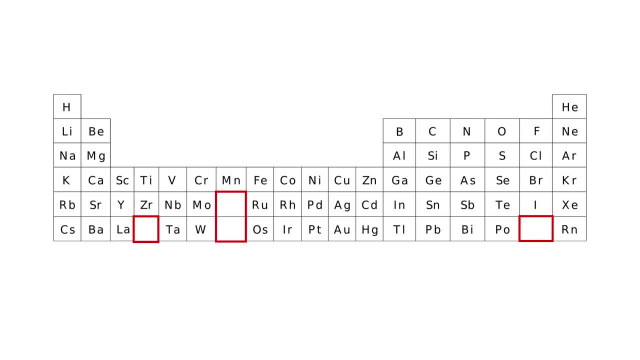 gaps in the table. Mendeleev said there must be elements that go in these spots and he predicted some of their properties. eventually, these elements were discovered with the properties precisely as expected, and now we have all the metals, metalloids and non-metals organized nicely. 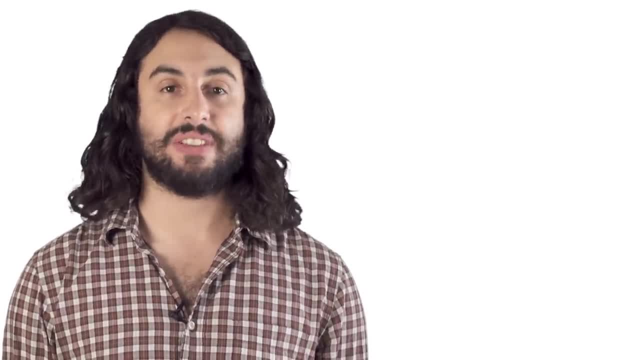 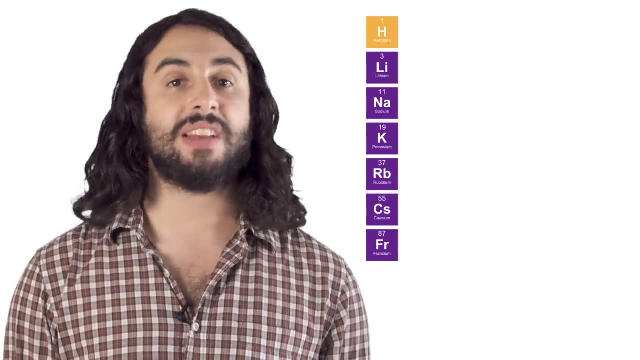 it wasn't known at the time, but the reason elements in the same group behave similarly is because they have the same number of valence electrons. look at group 1, for example. these elements all have one valence electron, or one electron in their outermost shell, as you. 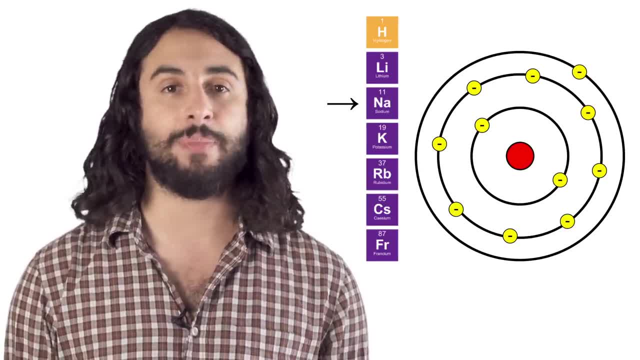 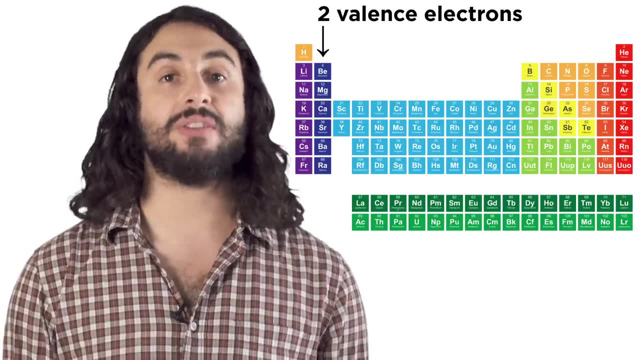 go down the table and n increases. you gain a shell each time. but whichever is the outermost shell, there is only one electron in it. every element in group 2 has two electrons in its outermost shell, and so forth. this simple fact determines: 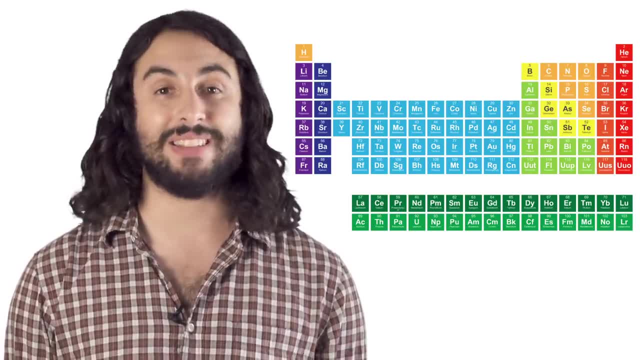 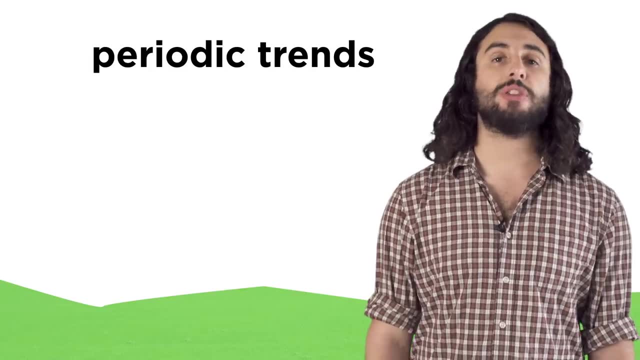 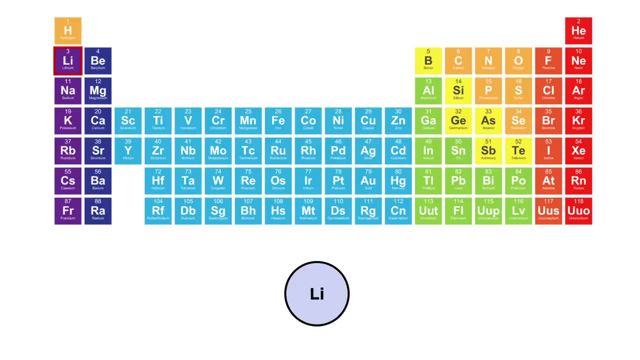 many characteristics about each element, in ways we will continue to see as we learn more chemistry. there are some periodic trends that we can recognize when we look at the table. the first one is atomic radius, or the size of the atom. as we proceed downwards on the table, atomic size increases because 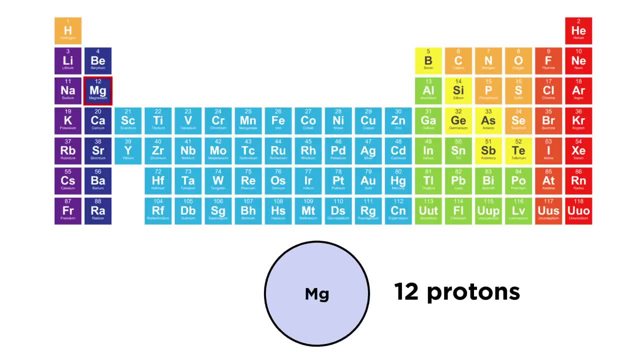 we add shells. as we go to the right, atomic radius decreases because we are moving within a shell and each element to the right has one more proton in the nucleus than the last, so there is a stronger electromagnetic attraction felt by the electrons and the 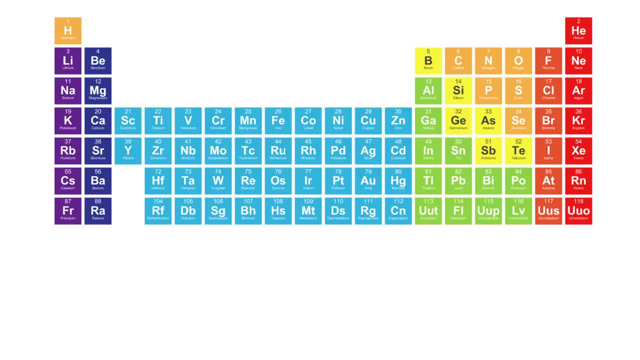 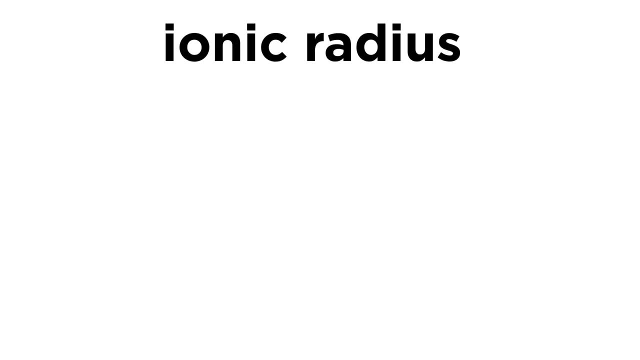 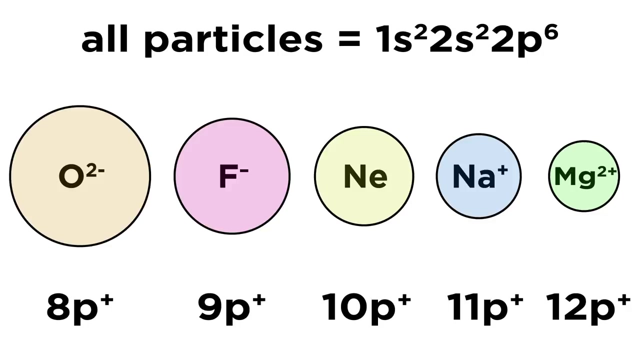 radius shrinks, that means overall atomic radius increases going this way. on the periodic table ionic radius is a little different. electrons repel each other, so adding an electron makes an atom bigger, taking one away makes it smaller. ions with the same electron configuration will have their radii decrease as the 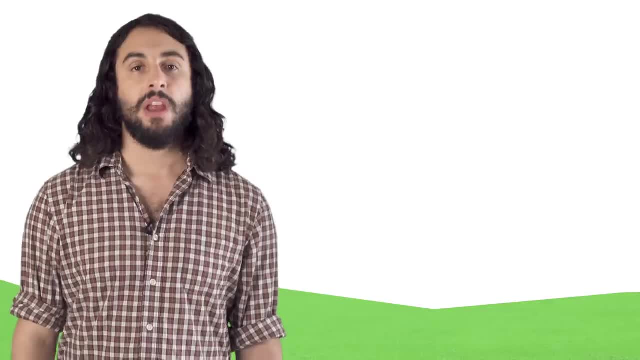 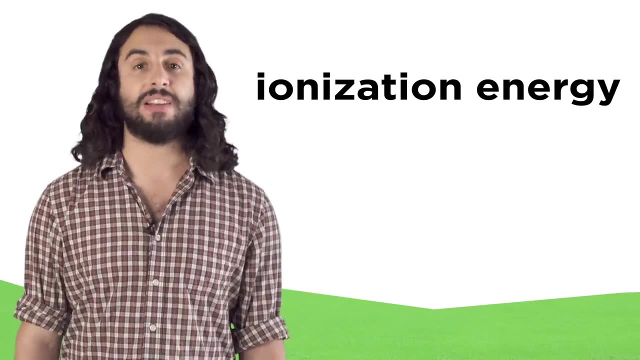 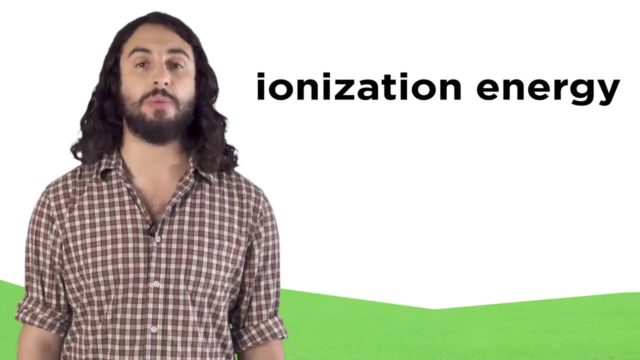 atomic number increases. next we look at ionization energy. this is the energy required to remove an electron from the atom. it will always be an electron in the outermost shell. the electromagnetic force that attracts the electrons to the protons drops off very quickly with distance, so the farther 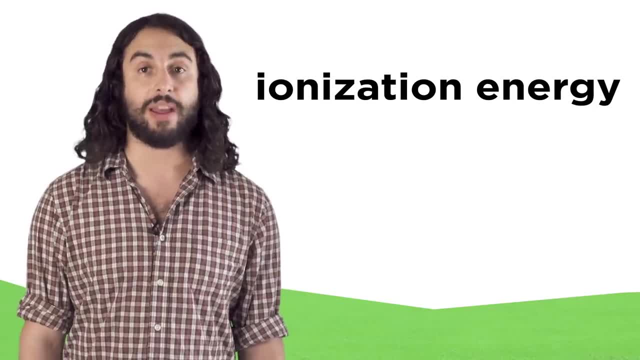 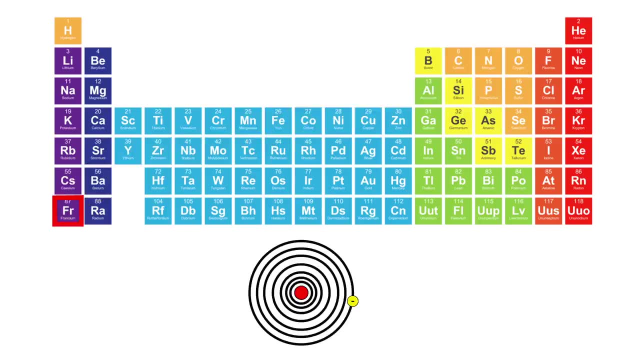 away an electron is from the nucleus, the easier it is to pull it away. this means the ionization energy trend is precisely the opposite of the atomic radius trend. francium, a very large atom with only one valence, electron, will be easy to ionize. 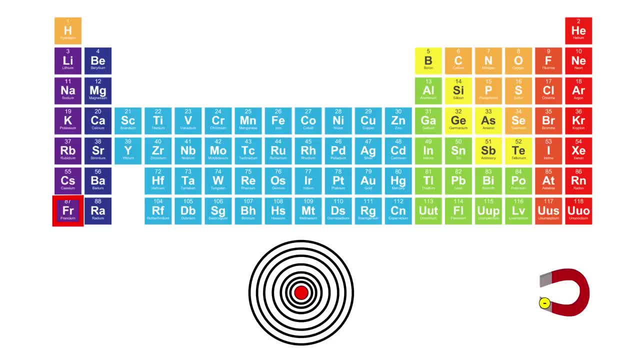 because the electron is so far away from the nucleus and atoms like to have their outermost shell completely full. losing the electron means this shell is gone and the one below is completely full. so elements in group one will easily lose one electron. looking at the opposite corner, with helium there is only one. 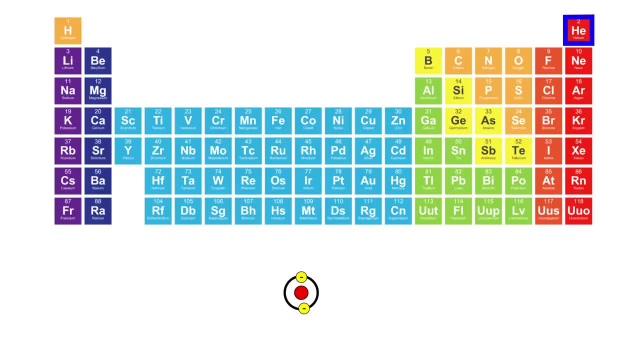 shell, so the electrons are very close to the nucleus and the shell is full, so it is very stable. for this reason it requires much more energy to ionize helium, so the ionization energy increases going this way. on the periodic table elements. 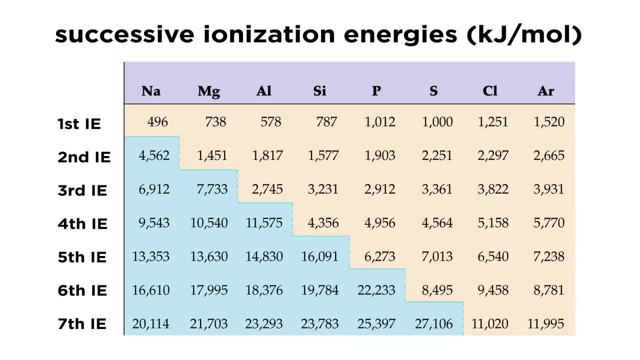 can have successive ionization energies. for removing more than one electron, a second ionization energy will always be greater than the first and continue to increase from there, since the more electrons you remove, the less stable the atom becomes. an element will have. 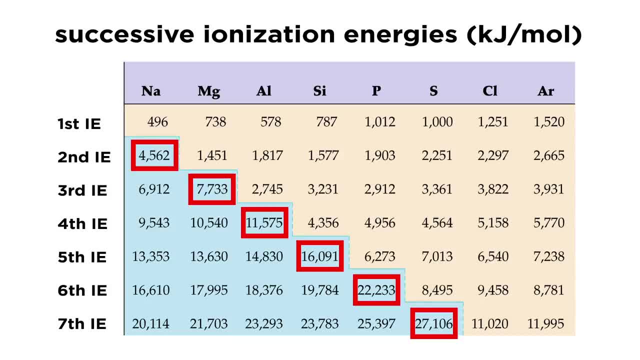 a huge jump in ionization energy after you take the last one in a shell, because then you jump to the noble gas electron configuration from the previous shell which is full, so it really won't want to give up any more electrons there are. 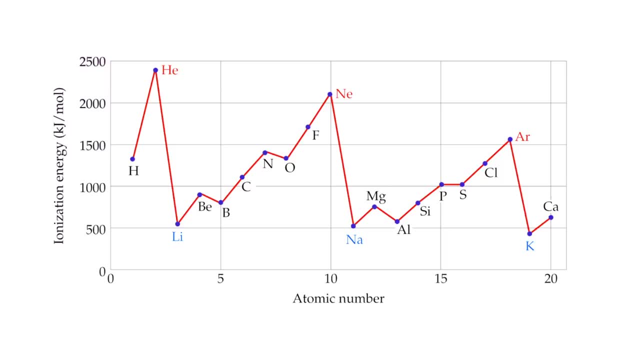 just a couple exceptions to the ionization energy trend, but we can rationalize them. look, for example, at the second row from lithium to neon. the ionization energy should increase each time we add a proton to the nucleus and the radius contracts a little, but something like oxygen which dips. 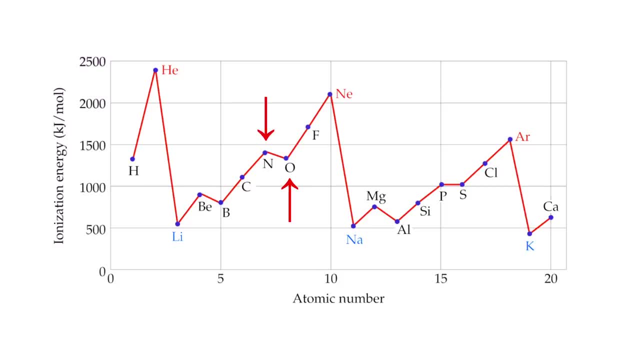 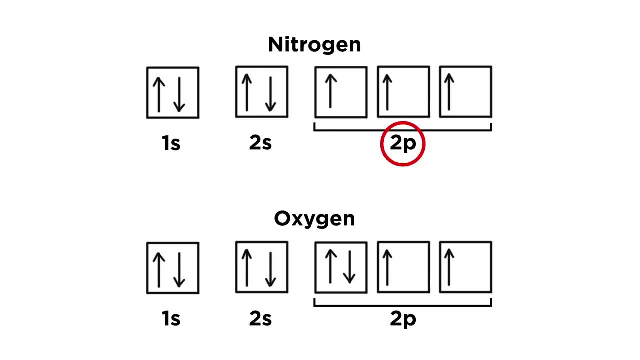 downwards from nitrogen's ionization energy does so because of orbital symmetry. here is nitrogen's orbital diagram, as well as oxygen's notice that nitrogen's two p orbitals are precisely half full. this gives nitrogen a special stability, just like elements that have a full outermost shell. if nitrogen loses an electron, it loses that. 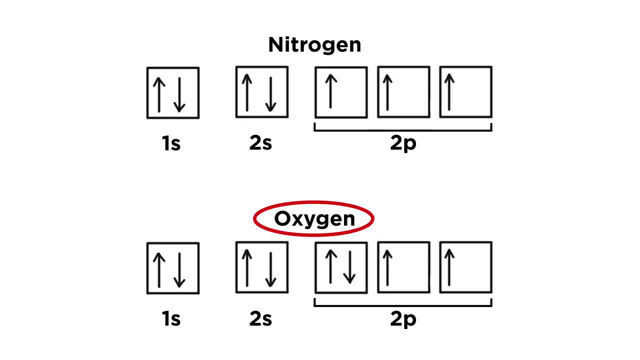 special stability. but if oxygen loses an electron, it will gain that special stability. that's why oxygen's ionization energy is a little bit lower than nitrogen's, even though oxygen has one additional point. all deviations from the ionization energy trend can be explained by. 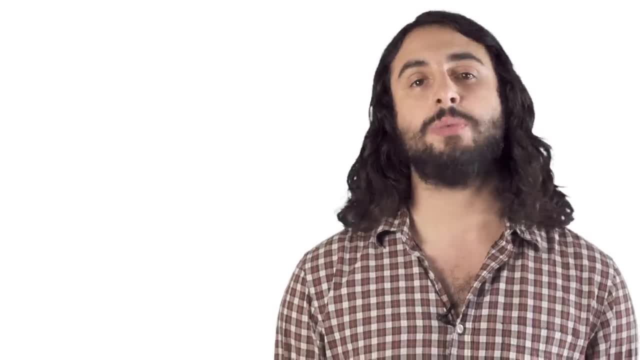 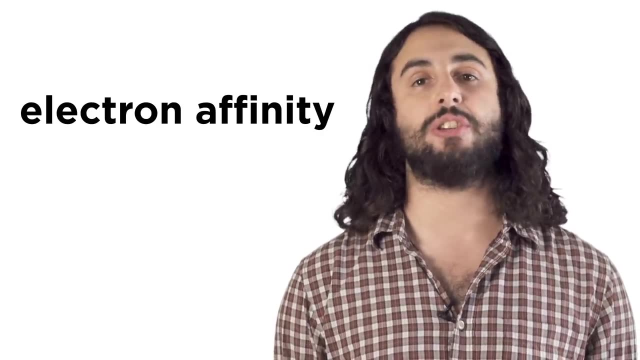 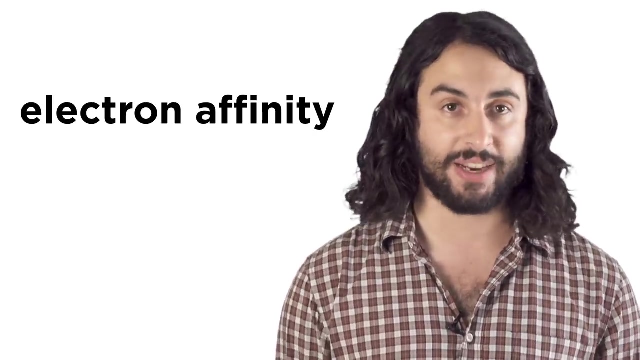 discrepancies in orbital symmetry like this one. next, we will look at electron affinity. this is exactly the opposite of ionization energy, since ionization energy is how much energy you need to remove an electron, and electron affinity tells us how much an atom wants to gain an electron, disregarding the noble gases. 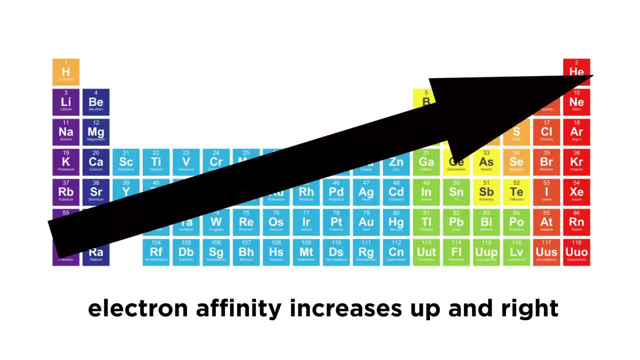 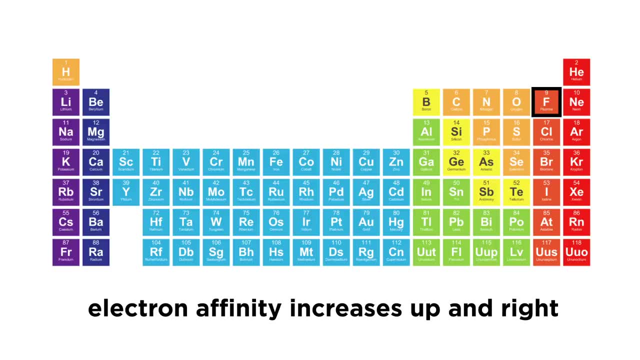 as their shells are full, electron affinity increases. this way, fluoride- fluorine- has the highest electron affinity because if it gains one electron it will have a full shell or a noble gas-electron configuration. looking at the opposite corner, these elements don't want to gain electrons, they would rather lose them. exceptions to: 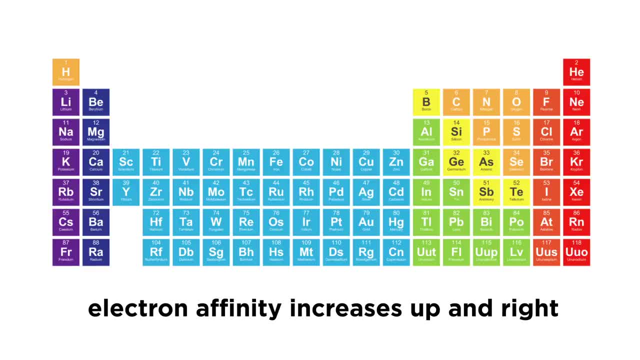 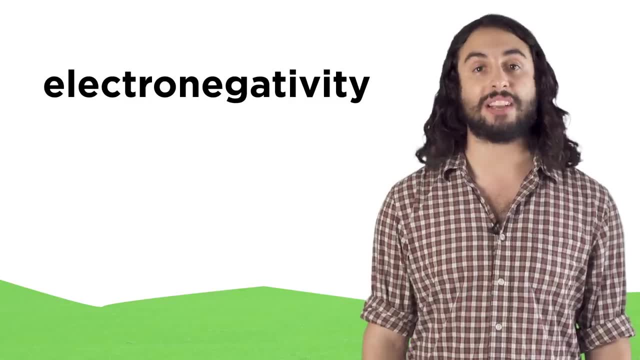 this trend happened for exactly the same reasons as the exceptions to the ionization energy trend. lastly, we want to look at electronegativity. this is the ability of an atom to hold electrons tightly. it will increase this way because a smallее electron affinity is more likely. 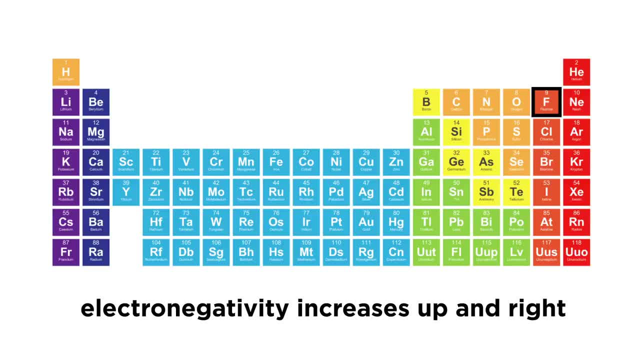 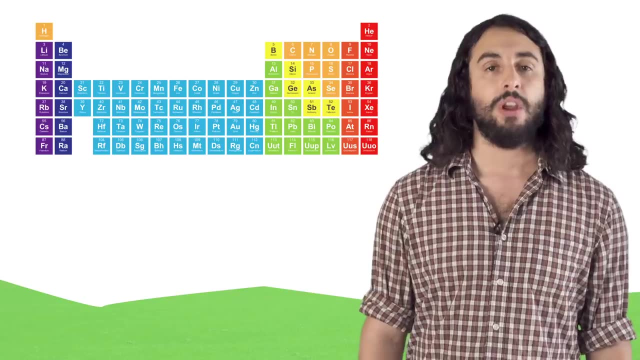 atom like fluorine, with more protons for its energy level or a higher effective nuclear charge, will hold electrons best. again, we will disregard the noble gases for this trend. electronegativity will be important in the next clip where we learn about chemical bonds. so the trends to remember are atomic radius, which goes